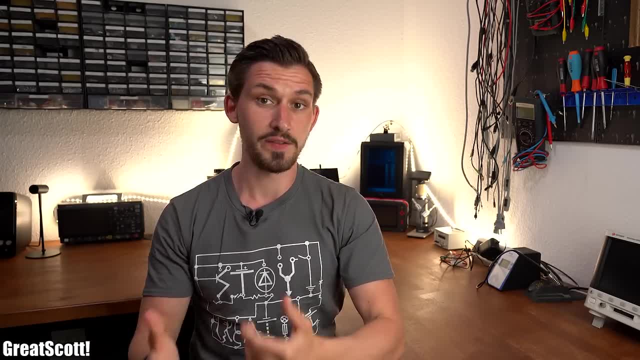 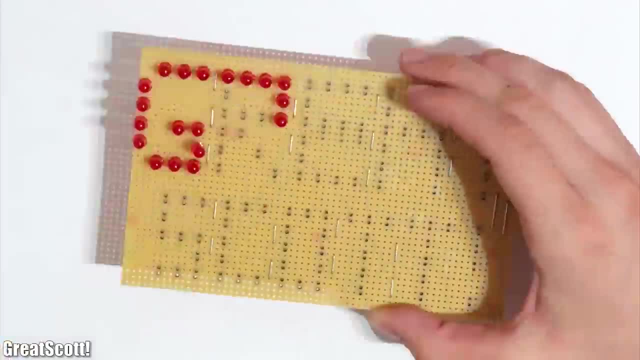 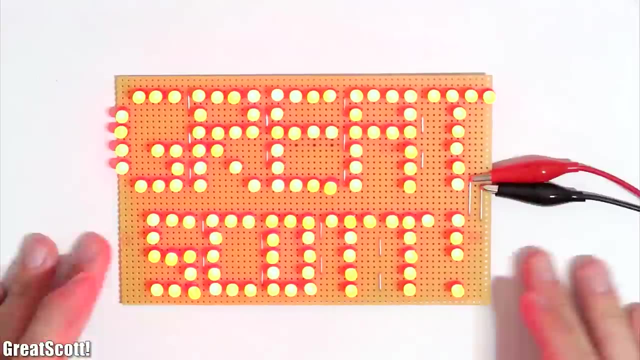 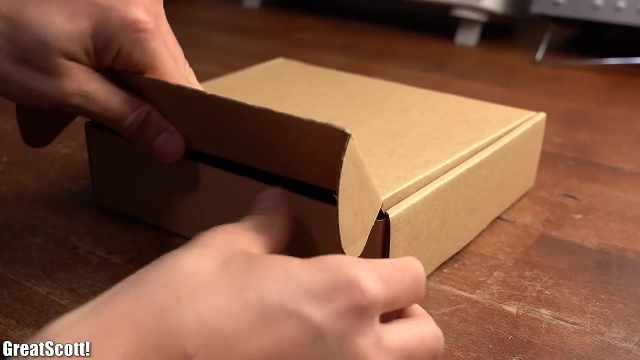 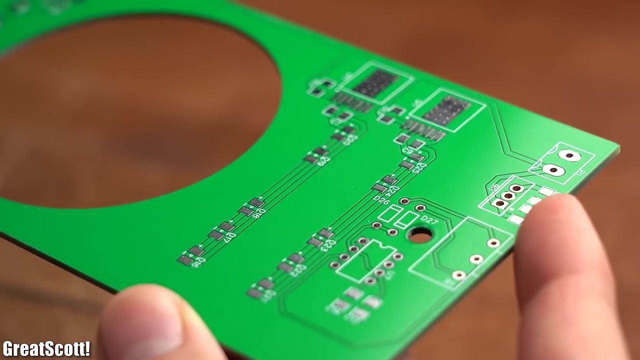 for example, solder, since that would be a topic for another video. Now, with that being said, let's get started. This video is sponsored by JLCPCB, from who I just received new PCBs that I actually ordered not even a week ago, So feel free to try out their awesome PCB service and fast delivery times today by uploading. 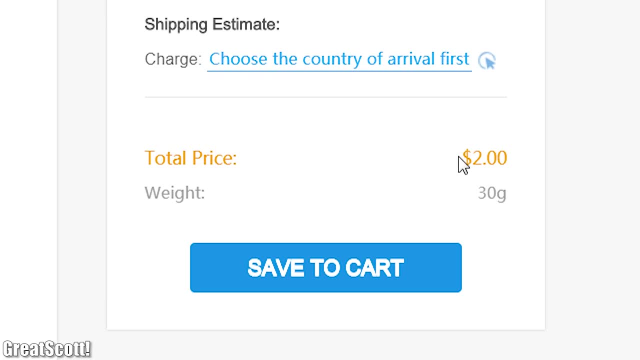 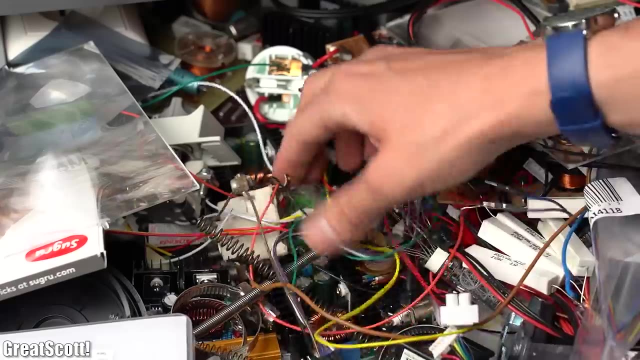 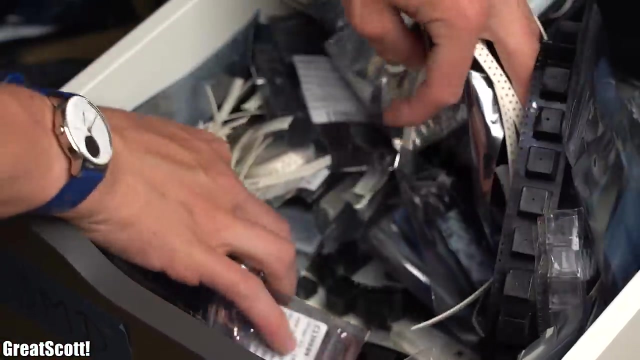 your Gerber files and get 5 PCBs for just $2.. Before we talk about electronics components, I would like to mention that shoving them all in one drawer is not recommended. Since you can get a lot of electronics components, you can never find what you are looking for when you are in a hurry. Instead, I recommend. 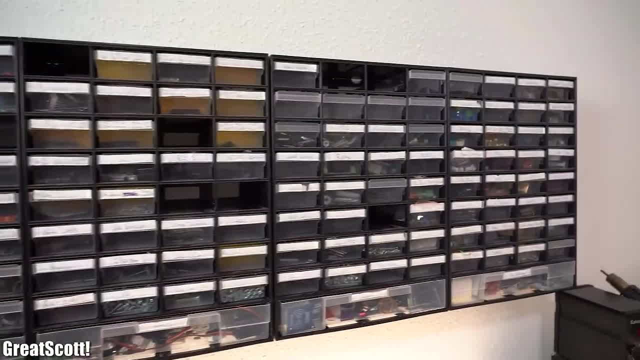 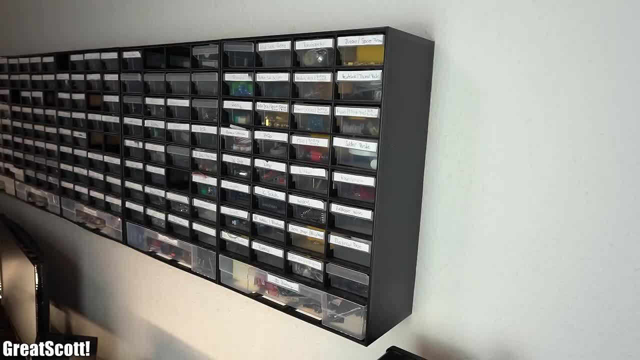 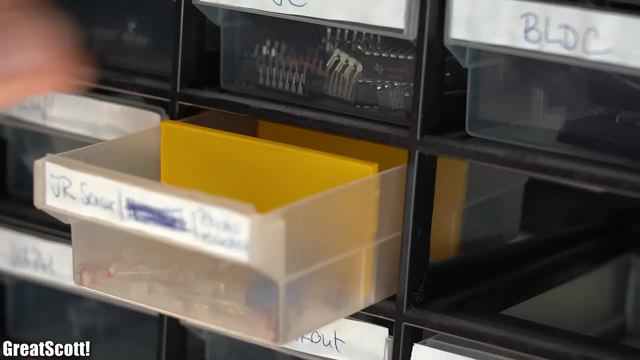 these wall mounted component storage boxes, of which I have plenty Now. granted, they are not the cheapest option, but they are super simple to mount, their drawers can be divided and they are easy to label, which makes finding a specific component very easy. With that being said, let's start off with the most basic passive components, which are: 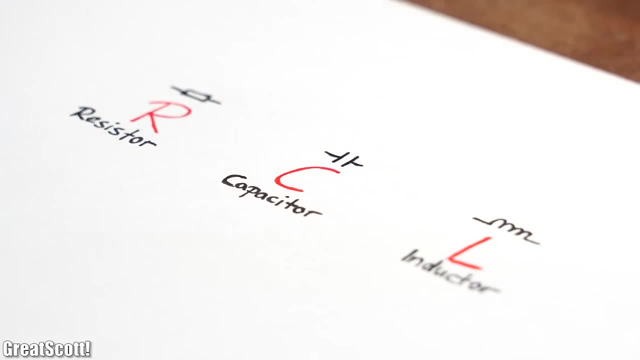 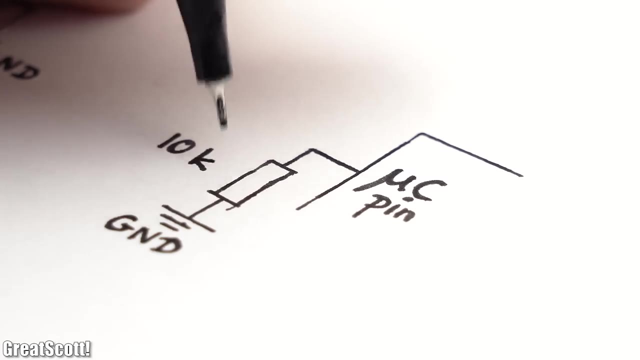 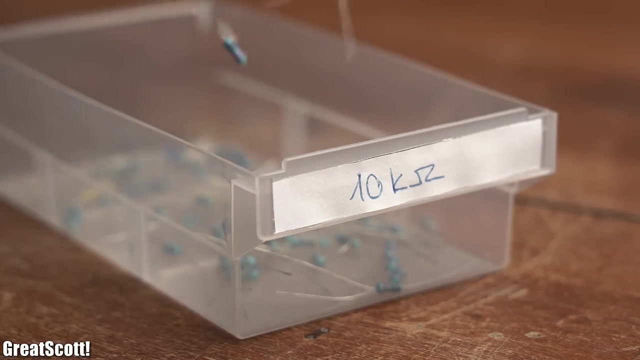 resistors, capacitors and inductors. beginning with resistors, Their main job is to limit the current flow and pull a certain part of a circuit to a voltage potential, which is why you should always have tons of 10kΩ resistors. But besides that, I also highly recommend such 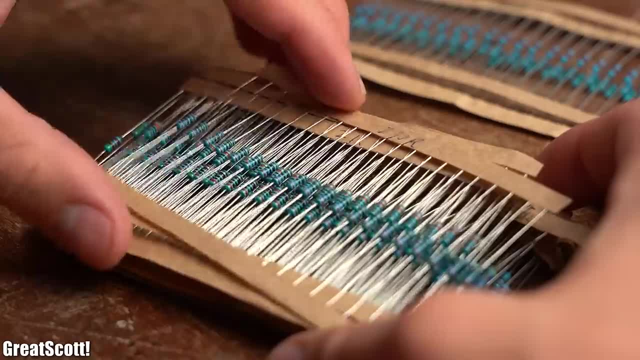 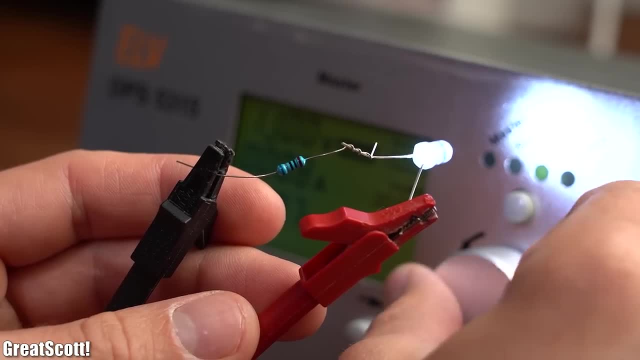 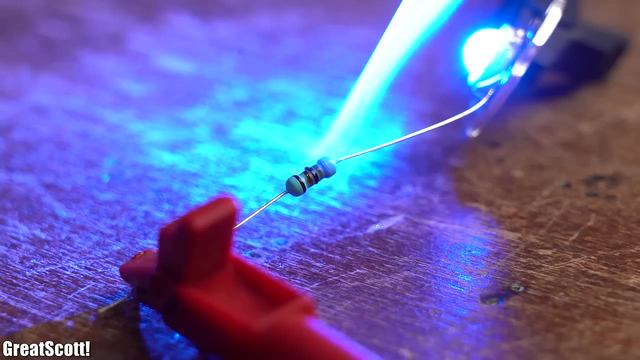 a ¼W metal film resistor kit which basically comes with all the values you could possibly need for a circuit, And a ¼W is plenty for normal projects. Of course, if you want to limit the current of a high power LED with them, then you might. 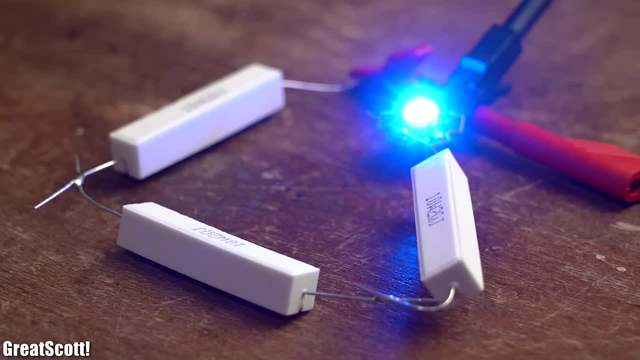 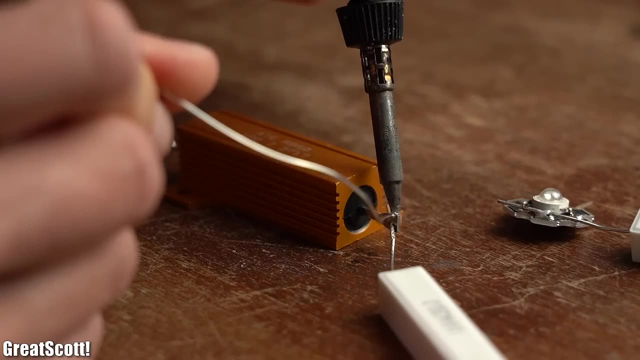 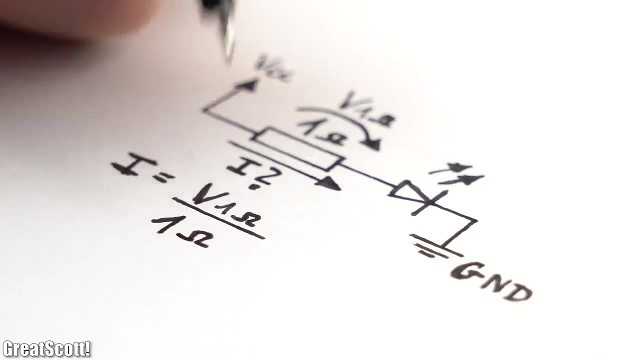 run into problems, But if you got a specific project in mind, then you can always get yourself a specific power resistor fairly easy. The only power resistors you should have laying around are 1Ω ones, because you can place them in series to your load and thus use them as a shunt to monitor the current flow. 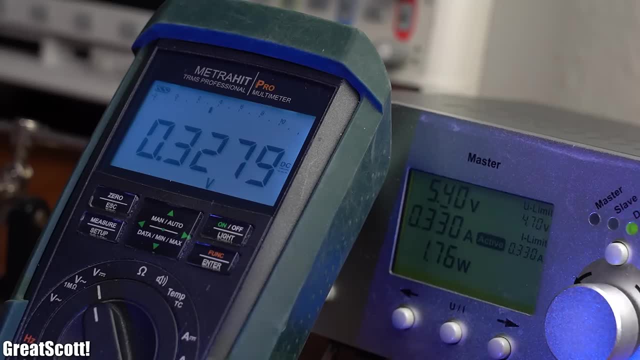 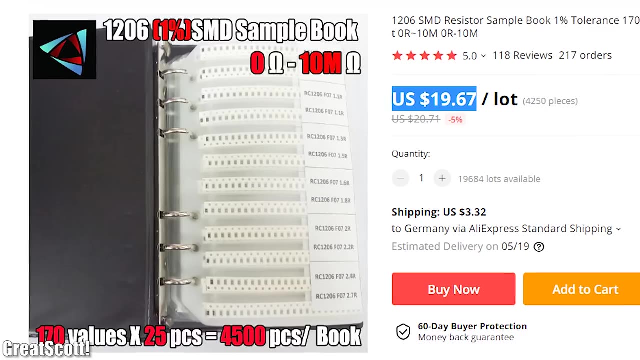 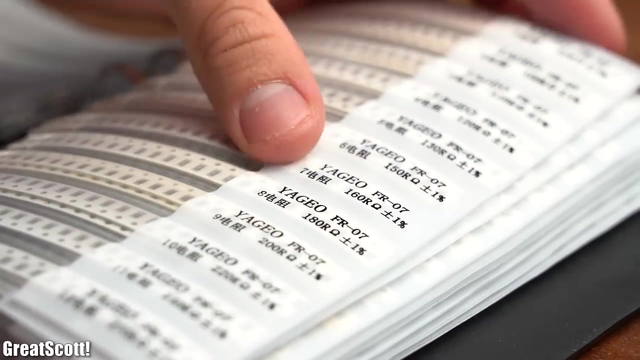 And last but not least for resistors, since I am also getting more and more into SMD circuits, I recommend such a 12-06 SMD resistor sample book, in which you can quickly find the desired resistor value and the 12-06 size is still pretty easy to solder by hand. 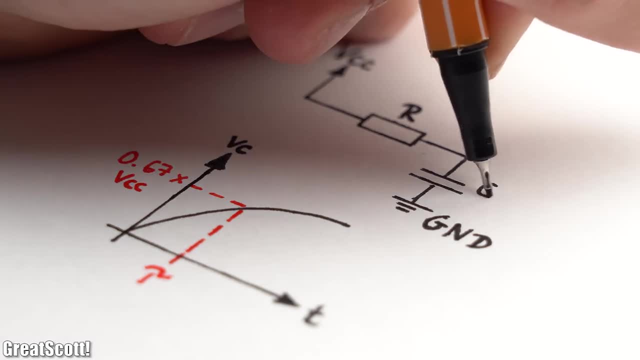 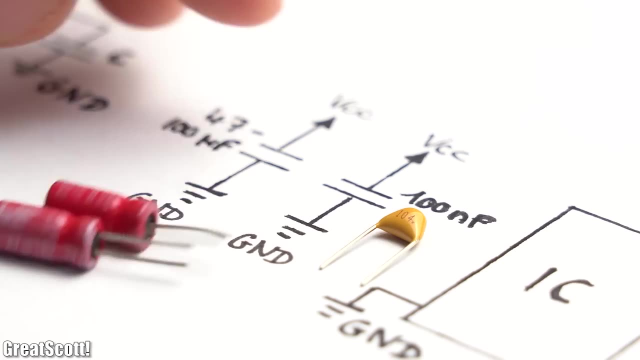 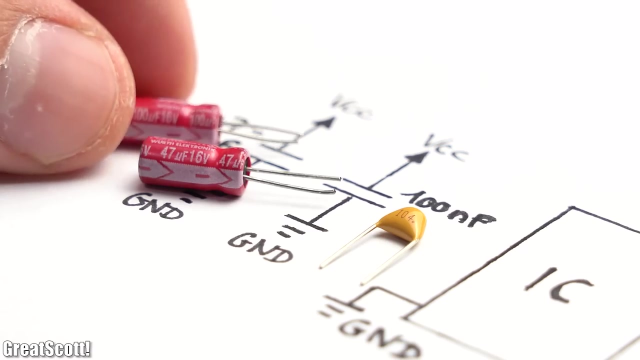 Next, we got capacitors which are not only useful for creating RC time circuits, but also act as energy reservoirs for decoupling purposes, Which is why 100nF ceramic capacitors and 47-100μF electrolytic capacitors are super. 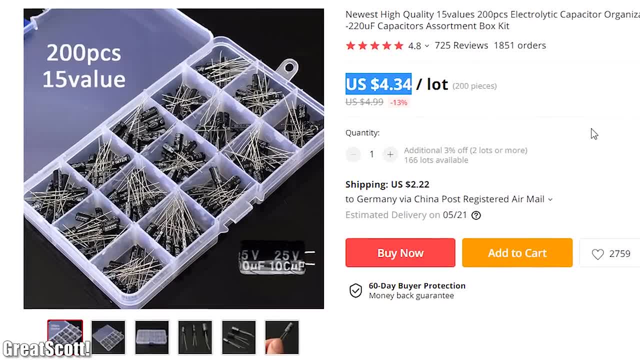 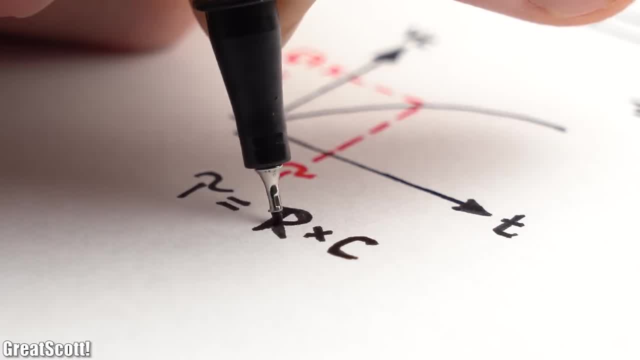 important, But it would be the best if you got one of those electrolytic and ceramic capacitor kits laying around, just in case you want to build up a specific RC time circuit. And once again for SMD circuits, I recommend a 12-06 SMD resistor sample book, in which 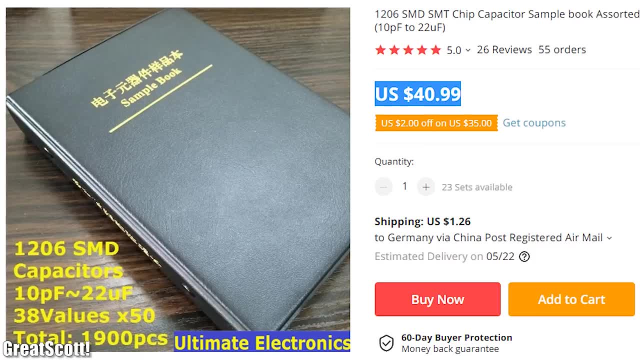 you can place them in series to your load and thus use them as a shunt to monitor the current flow And, last but not least, for resistors. since I am also getting more and more into SMD circuits, I recommend such a 12-06 SMD capacitor book, in which you can quickly find the desired resistor value and the 12-06 SMD capacitor kit laying around, just in case you want to build up a specific RC time circuit, Which is why 100nF ceramic capacitors and 47-100μF electrolytic capacitors are super. 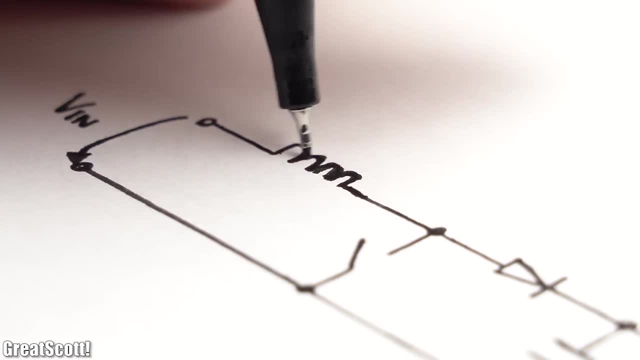 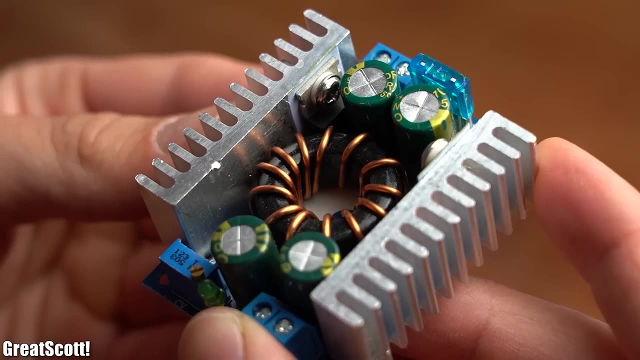 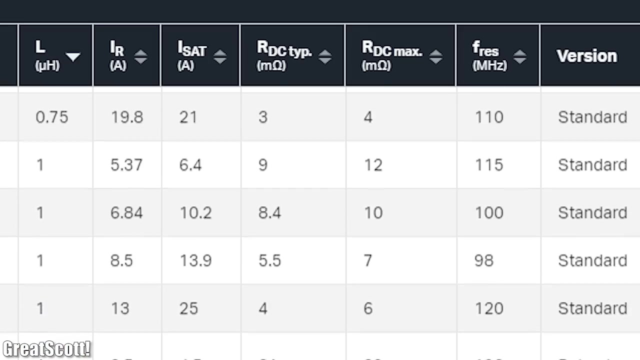 important. Last but not least, we got inductors, which are mostly used as energy storage devices, for switch mode power supplies or to build up filters. In the first case, your choice of inductor truly depends on what kind of power supply you want to build, and thus it is advised to search for specific ones when you know the 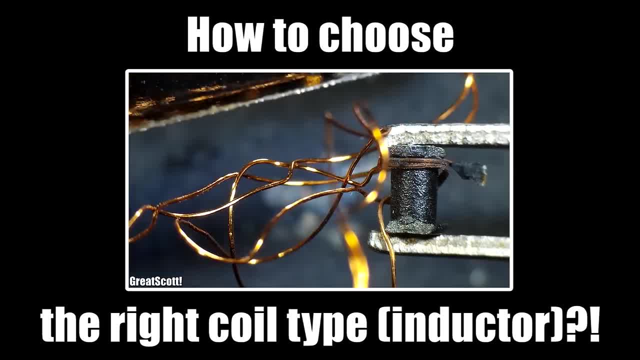 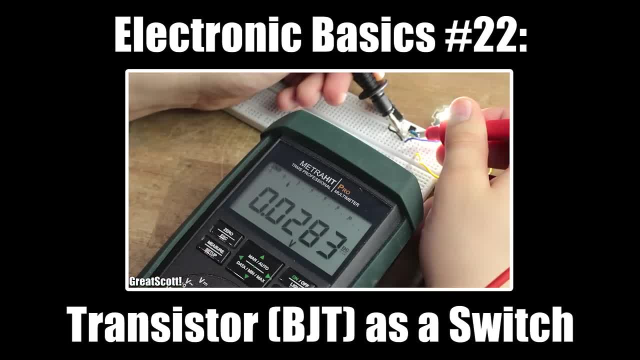 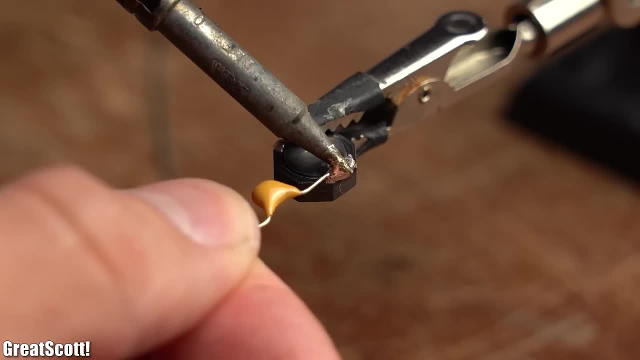 details of your circuit. But you should know that if you watched my video on how to choose the correct coil- And, by the way, you can find all of my existing videos- to the here mentioned components in the video description. Anyway, for building up filters on the spot, however, I would recommend such a power inductor: 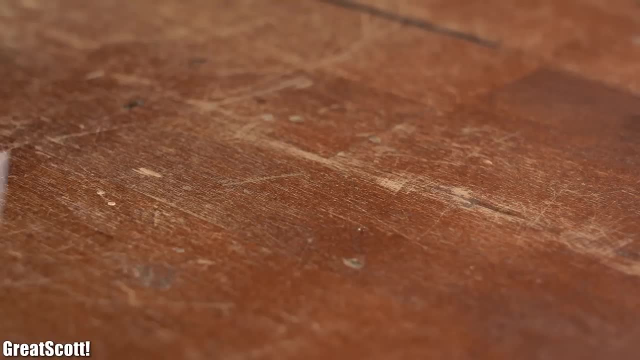 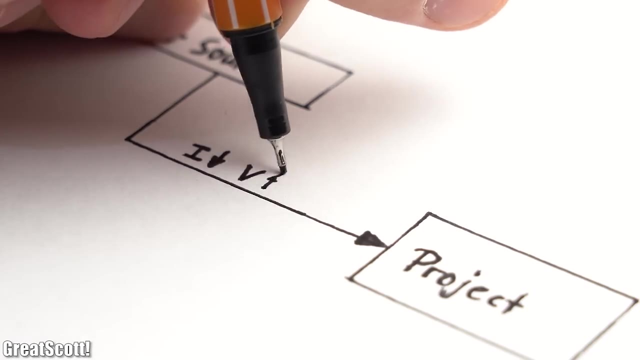 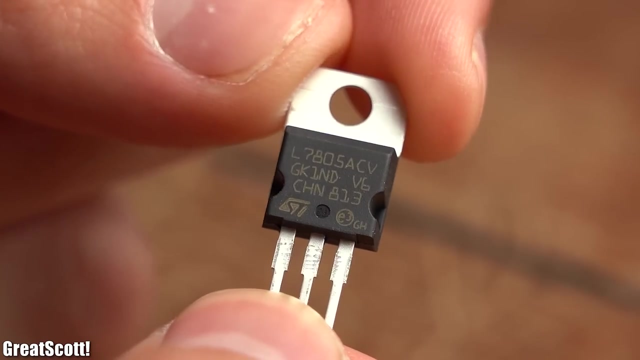 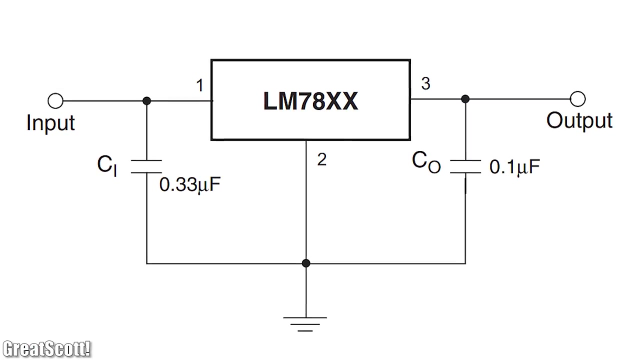 kit And with the basics out of the way, let's move on to regulating the input power to projects. For low current projects, Where you got a high input voltage and either require the common 5V or 12V, I would recommend either the LM7805 or the LM7812, which, according to the datasheets, are super simple to set. 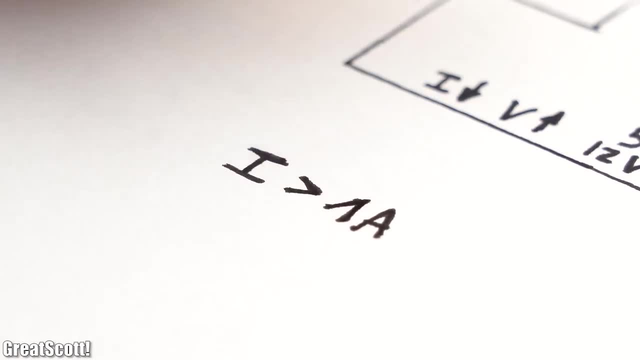 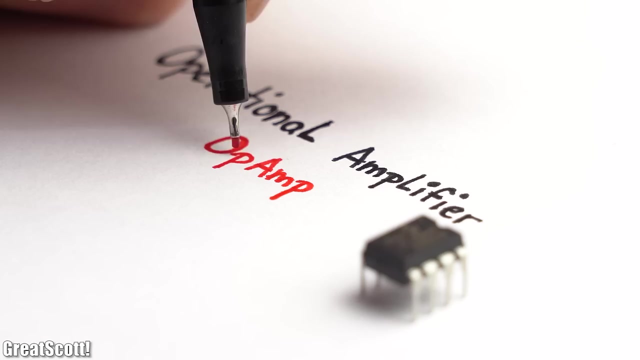 up. For a bit more current, demanding tasks, however, I would recommend the boost converter built around the MT3608 to step up voltages, or the buck converter built around the LM258 to step up voltages. The next essential component is the operational amplifier, or op-amp, which can not only like 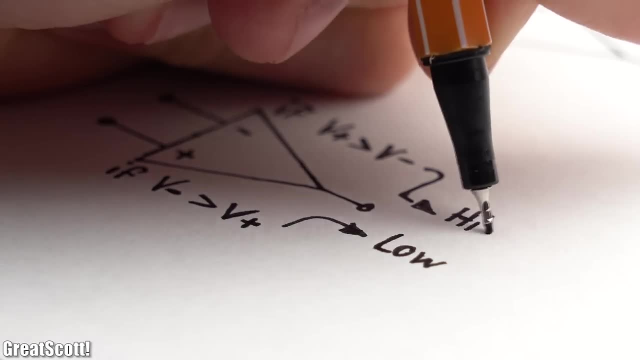 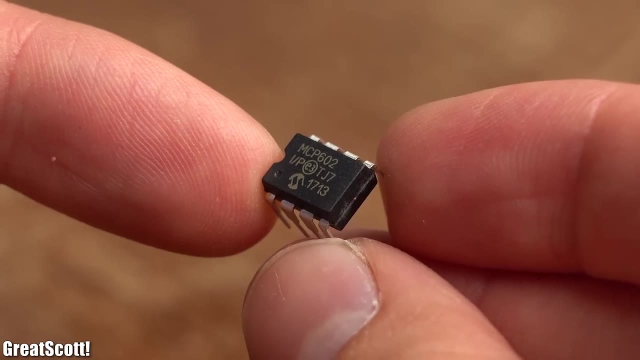 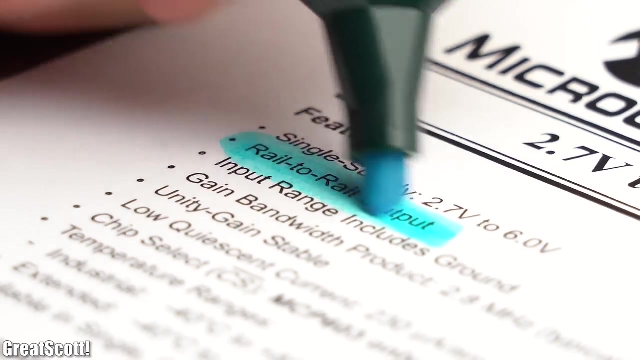 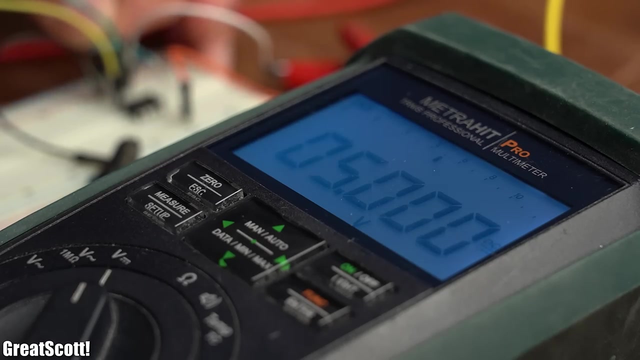 the name implies, amplify voltages, but can also be used as, for example, a comparator For 5V projects. I always go with the MCP602, which not only features two op-amp stages but also comes with a rail to rail output, Which means its output can swing almost completely up and down to the supply voltage limits. 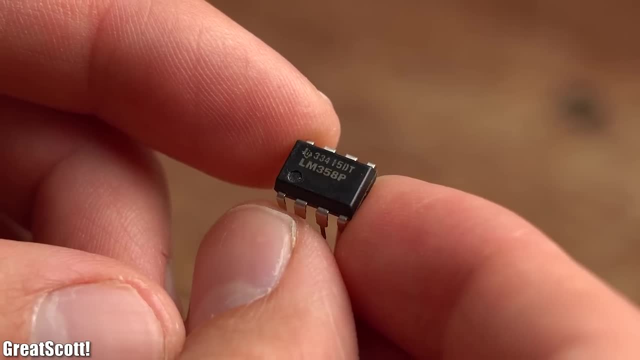 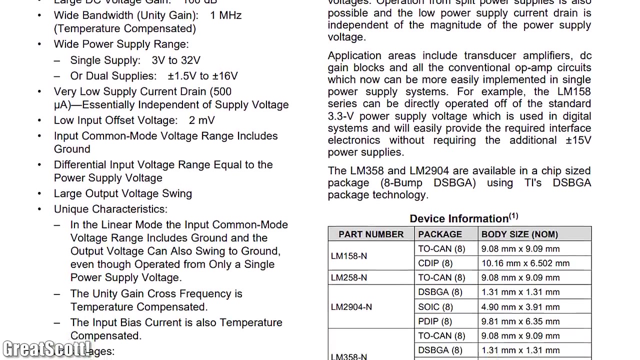 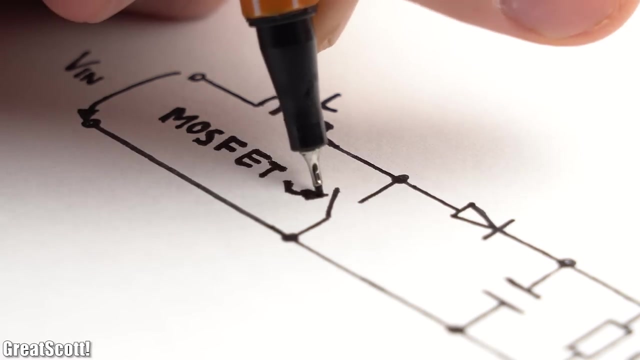 For 12V projects and beyond, I mostly go with the LM358, which is a pretty generic op-amp that always works for me. Next we got the MOSFETs, which are basically efficient electrical switches which can be used in switch mode power supplies or to basically switch things on and off. 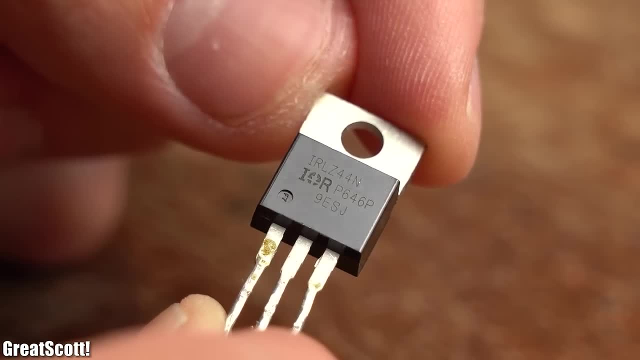 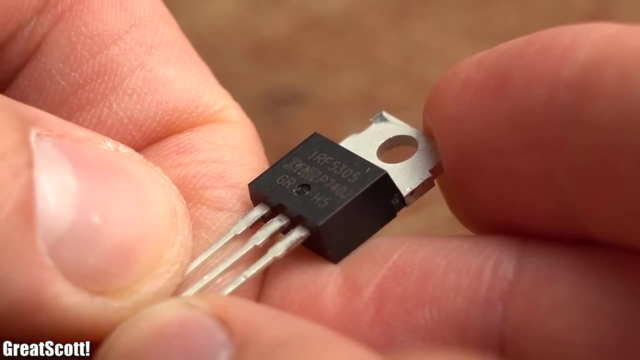 I would recommend the MOSFETs, which are basically efficient electrical switches which can be used in switch mode power supplies or to basically switch things on and off. I always go with the IRLZ44N N-Channel MOSFETs for low side switching or the IRF5305 P-Channel. 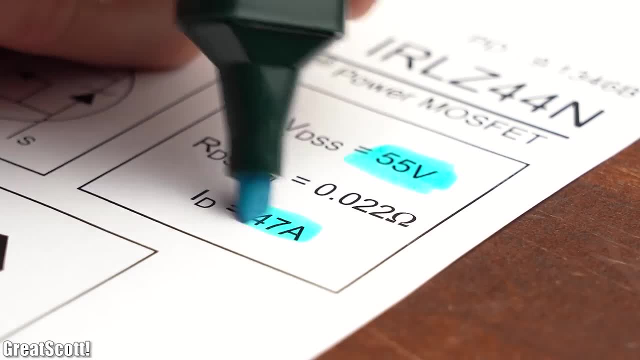 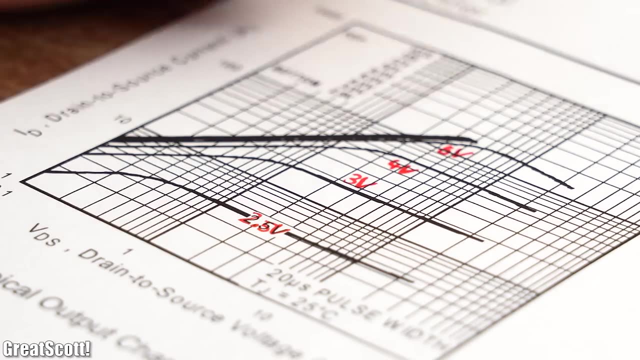 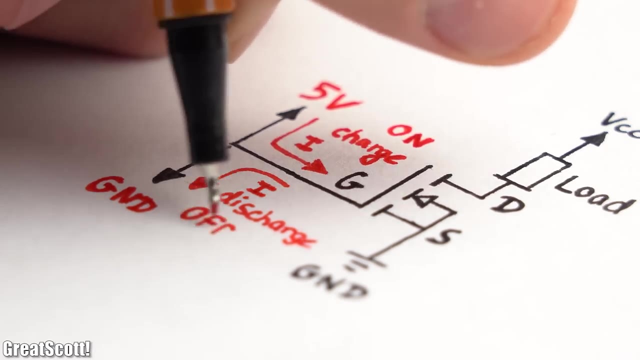 MOSFETs for high side switching. They both can handle high current and voltage values and are easy to drive with low level logic voltages. And speaking of driving, since it is always important to charge and discharge a MOSFET gate as quickly as possible, 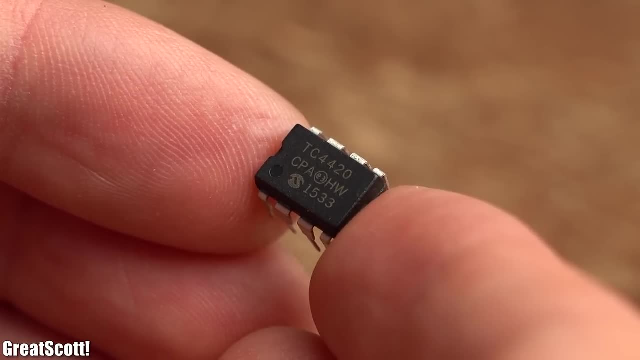 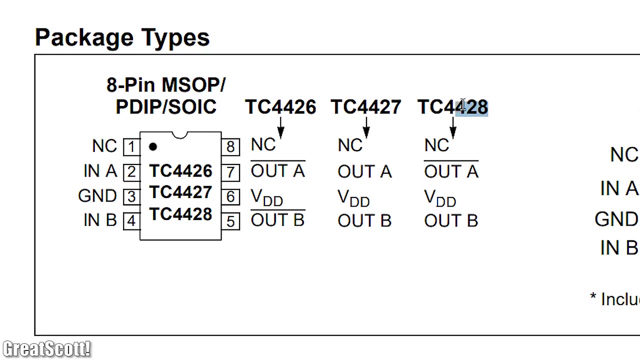 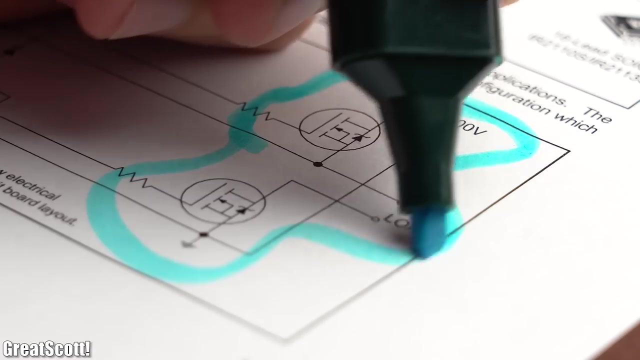 Make sure to wearorrover plugs. Stay tuned. TC4420 MOSFET Driver IC. or if you want to drive more than one MOSFET simultaneously, then the TC4428 IC or its siblings are your best friend. But let's say you want to build up a half bridge or full bridge with n-channel MOSFETs. 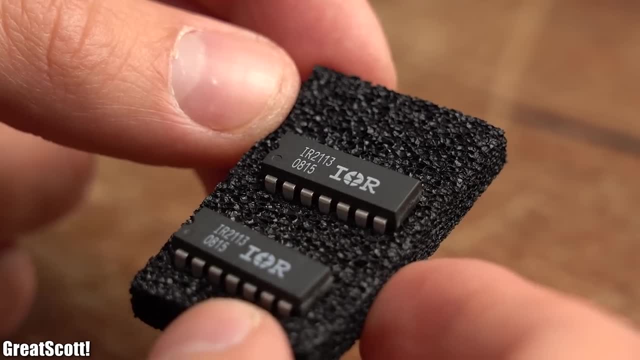 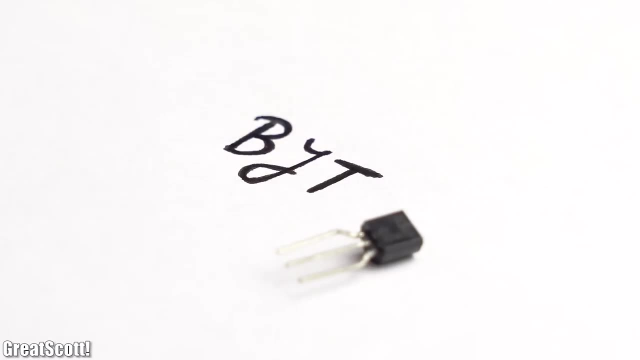 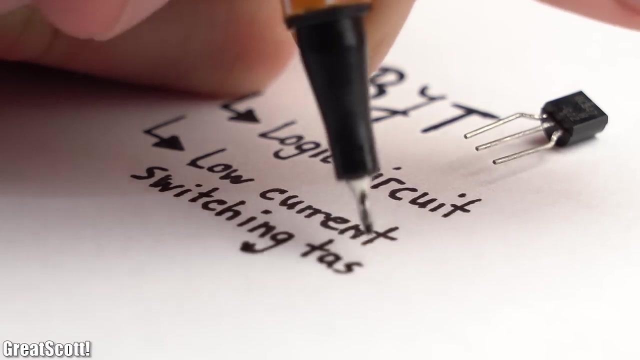 then I would recommend the IR2113 Driver IC, since it comes with a bootstrapping feature. Next, we got BJTs, which I pretty much only use when I want to build up a small transistor logic or do not want to waste a MOSFET on a low current switching task. 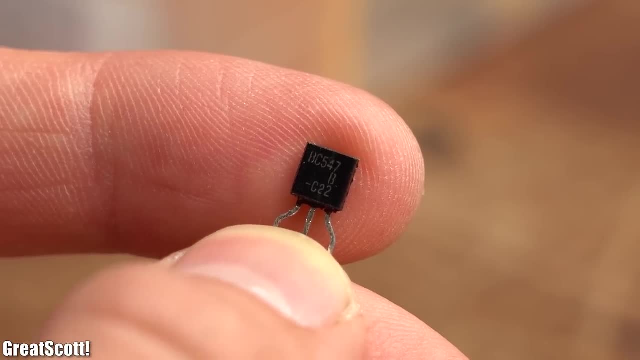 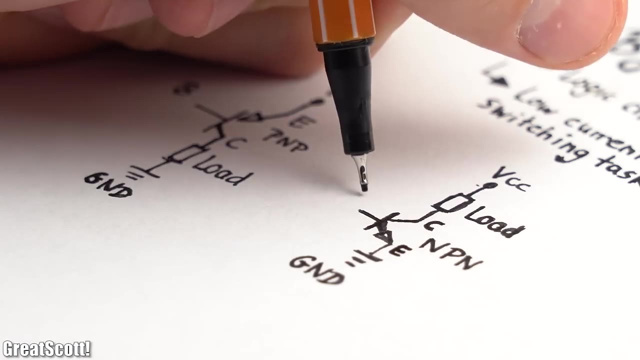 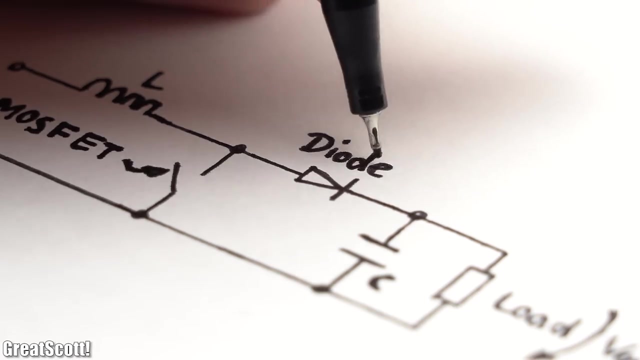 That is where I either use the BC547 NPN BJT or the BC557 PNP BJT, Depending on how the load is tied to the supply voltage. Next we got diodes, which are not only mandatory for switch mode power supplies but also for 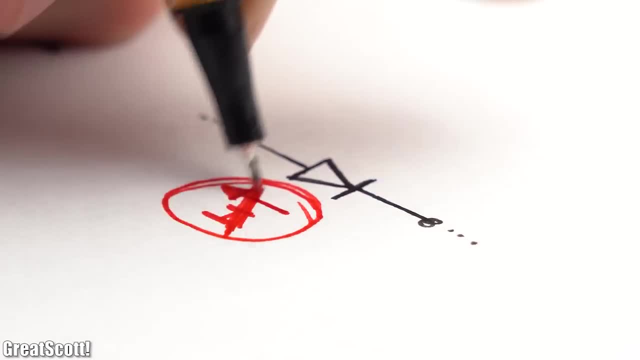 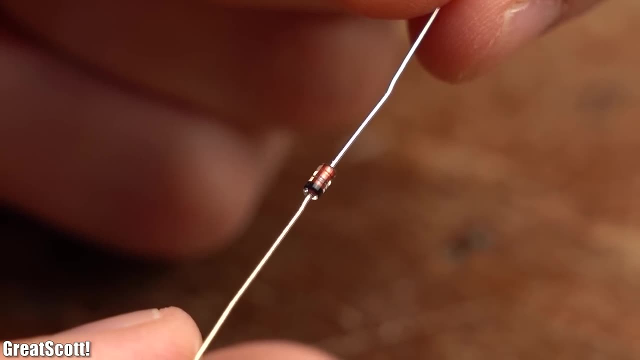 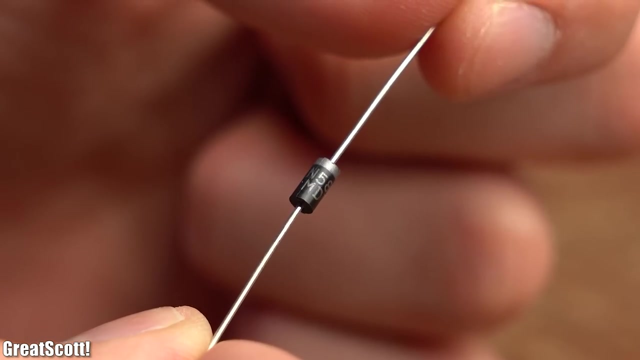 flyback purposes or, for example, reverse voltage protection For undemanding tasks, I use the general purpose 1N4148, or if I need a faster Schottky diode with a lower forward voltage drop Then the 1N58 or 1N4148. 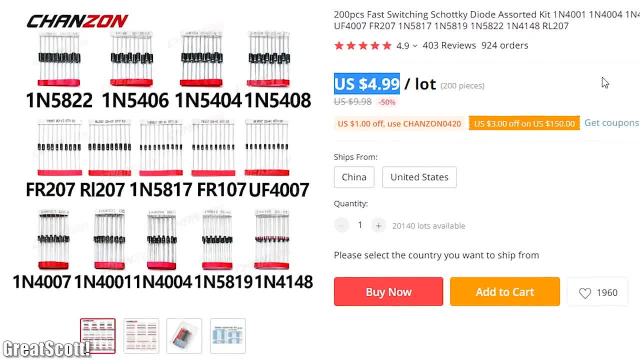 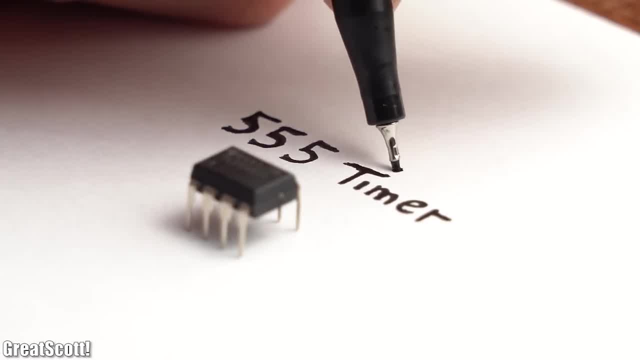 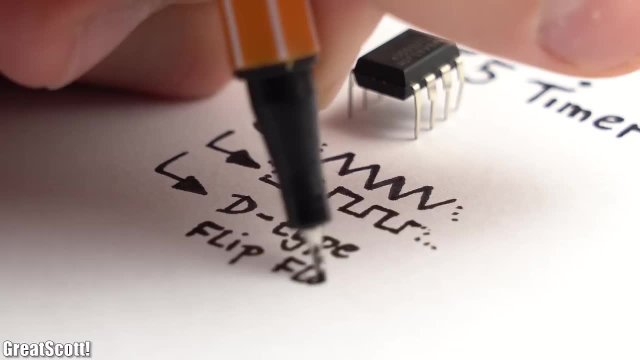 But if you get yourself such a kit, then you should have all the diodes that you could ever need. Next, we got the legendary 555 timer, which you can not only use to generate triangle and square wave voltages, but you can also use it as a D-type flip-flop. 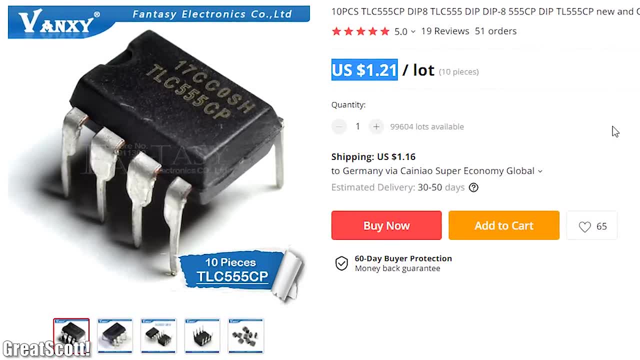 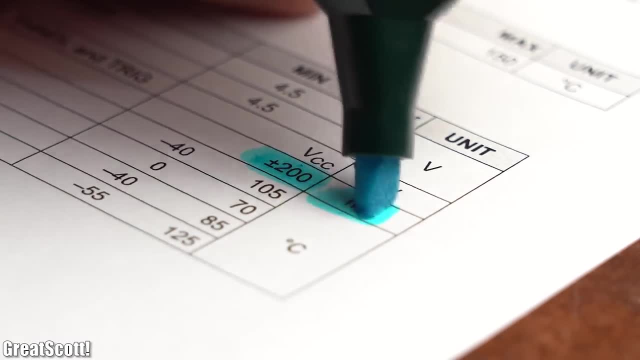 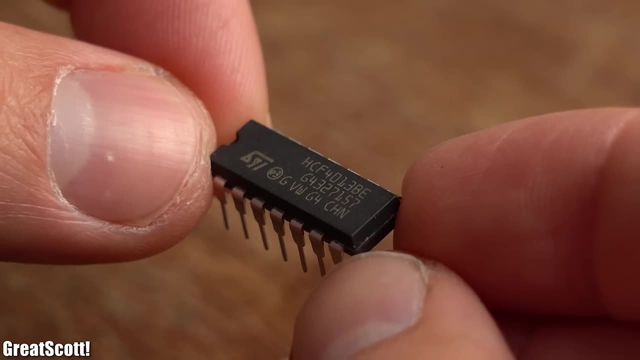 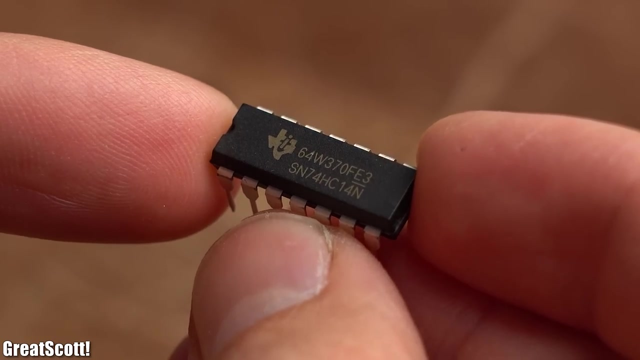 That is why I recommend having the TLC555 for demanding timing tasks and the NE555 for tasks where you need a bit more output current. Next, I thought about what logic ICs I mostly use And I have to say that, besides the HCF4013 D-type flip-flop, I only often use the 74HC14. 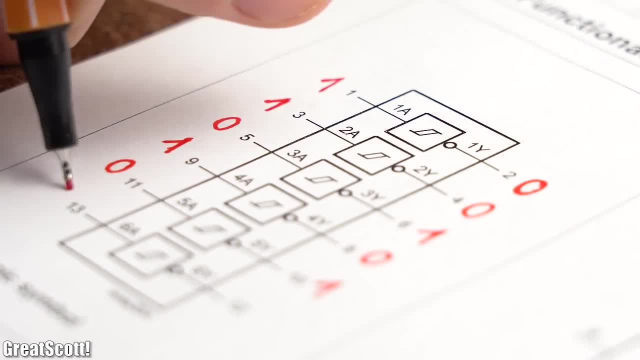 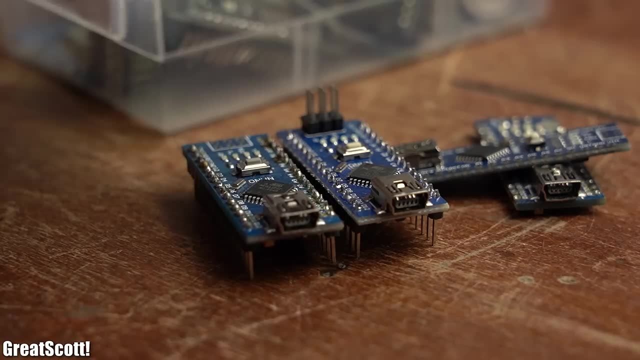 hex inverting Schmitt trigger IC which, like the name implies, can basically invert a logic signal. Besides that, I would always recommend having a couple of Arduino NICs. I would also recommend having a couple of hex inverting Schmitt trigger ICs which, like the name implies, can basically invert a logic signal. Besides that, I would always recommend having a couple of Arduino NICs. 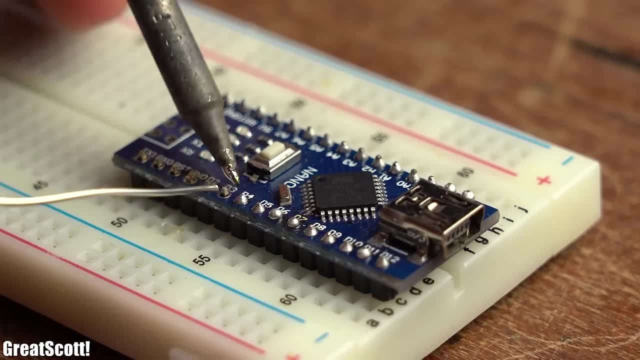 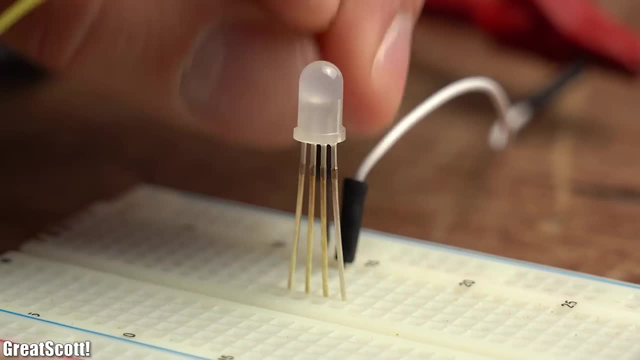 Since they are easy to setup and use- in just a few minutes- And there are thousands of applications for them. And, of course, we should not forget about LEDs, which are super handy to display a certain conditions of a circuit or to be the main attraction of the circuit itself.